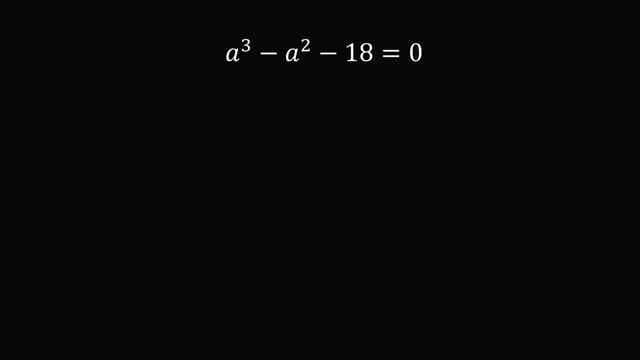 solve this problem. I'm going to show you how to solve this problem. I'm going to show you how to solve this problem. You don't need to see my other videos about values like 0,, 1 and so on until you get lucky. 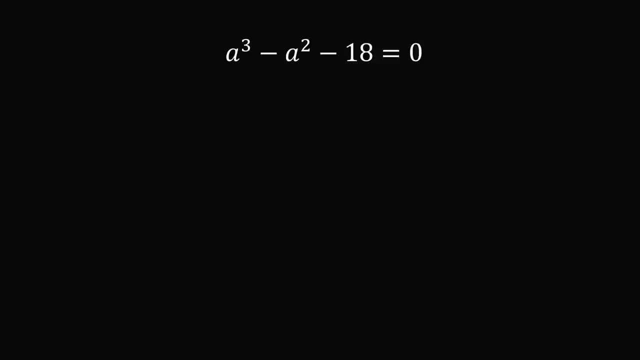 But there is a trick you should know: If you have a polynomial with integer coefficients, you should use the rational root theorem. So what this states is: you want to look for particular candidates which will be rational roots of this polynomial. So here's how it works: You take a look at the constant coefficient, which is 18, and then you take 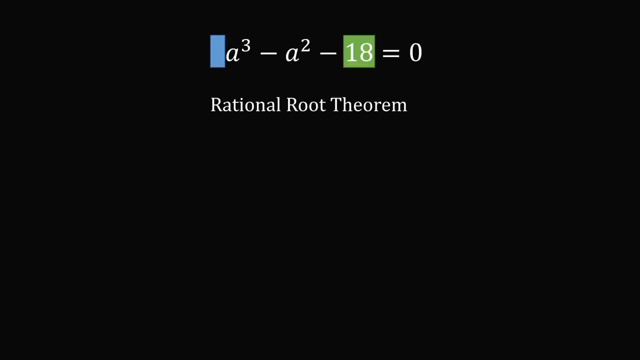 a look at the coefficient of the highest power. so in this case we want to take a look at the coefficient of a cubed. in this case the coefficient is 1.. so the candidates for roots of this polynomial will be plus or minus factors of the constant term 18 divided by factors of the leading coefficient. 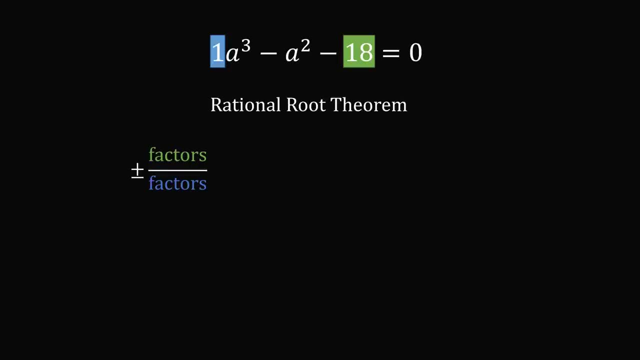 1.. so what are factors of 18? 18 factors into 1 times 18,, 2 times 9, and 3 times 6. so by the rational root theorem we look for plus or minus factors of 18, which will be 1, 2, 3, 6. 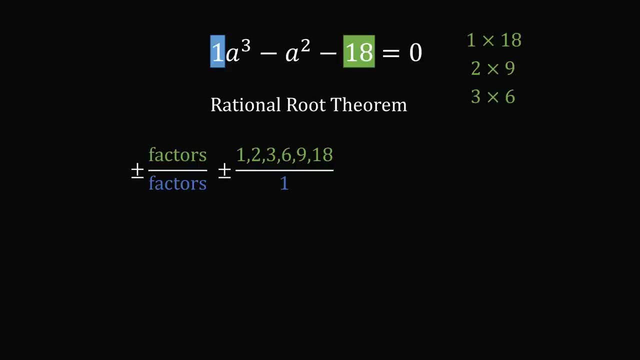 9 and 18 divided by factors of 1, one only has one factor, which is one. so this gives us candidate root Spear roots that we can check Plus or minus 1, 2,, 3,, 6,, 9, 18.. We don't need to check for 0.. We don't. 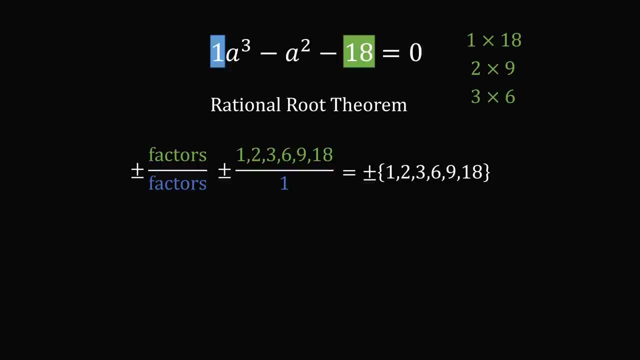 need to check for 4.. If there's a rational root, it'll be one of these candidates. So we'll just start checking. Let's try. a is equal to 1. We substitute in and we see this is not a 0 of the. 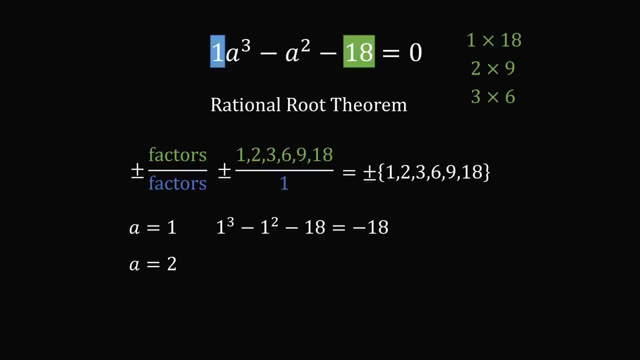 equation We can try: a is equal to 2, and once again we get unlucky. But what about a is equal to 3?? We get lucky. 3 cubed minus 3, squared minus 18, is equal to 0.. So we found a root of this. 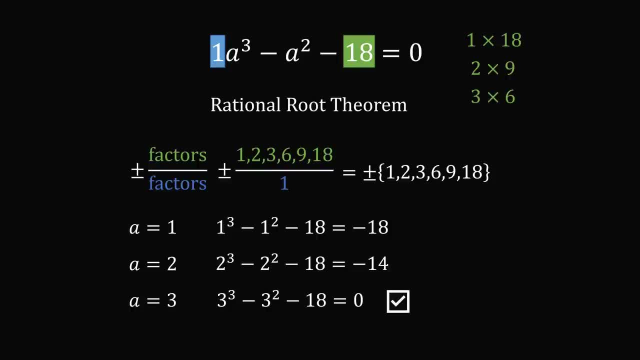 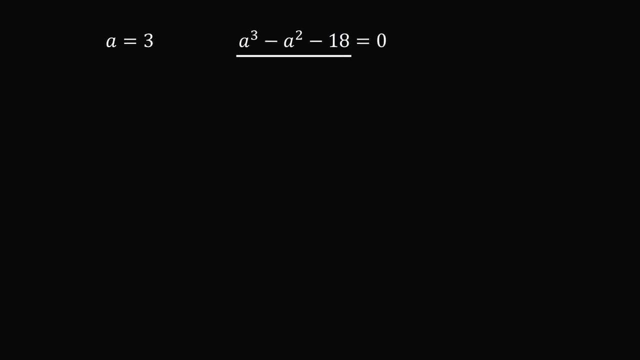 equation. Now we can simplify matters tremendously. Since a is equal to 3 is a root of the equation. a minus 3 will be a factor of the polynomial. So we will use polynomial long division. We take a cubed minus a squared. 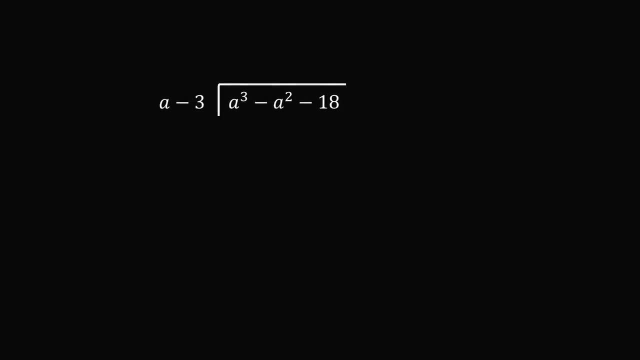 We take a squared minus 18, and we divide it by a minus 3.. Now when you do polynomial long division, you want to have all of the placeholders set. We don't have any coefficient for the linear factor, so let's just insert that We want 0 times a. So now we're all set. So first we want to eliminate. 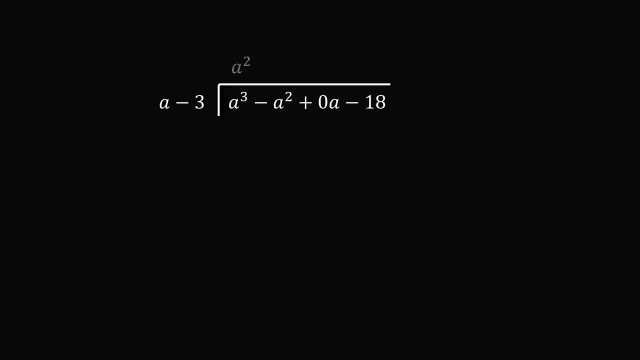 the a cubed term. So we need to multiply a by a squared. So we take a squared multiplied by a minus 3, and this is equal To a cubed minus 3 a squared. We will subtract this from the original polynomial and we have to. 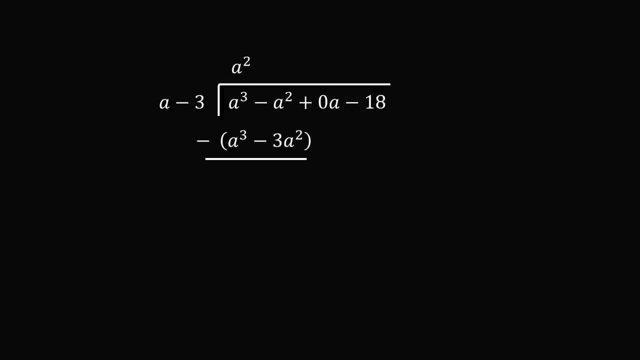 be careful about the opposite of negative. 3 a squared will be plus 3 a squared, So we end up with 2 a squared. Now we drop down the 0 multiplied by a. Now to eliminate 2 a squared, we need to. 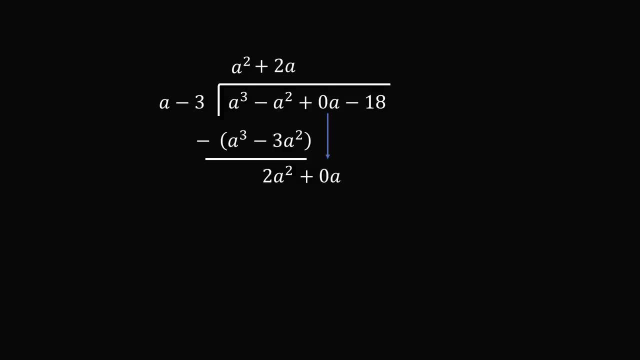 multiply by 2 a. So we add 2 a here. then we take 2 a multiplied by a minus 3. This works out to be 2 a squared minus 6 a. We want to subtract this entire term. This works out to be 6 a. We then bring down negative 18.. So to eliminate 6 a, 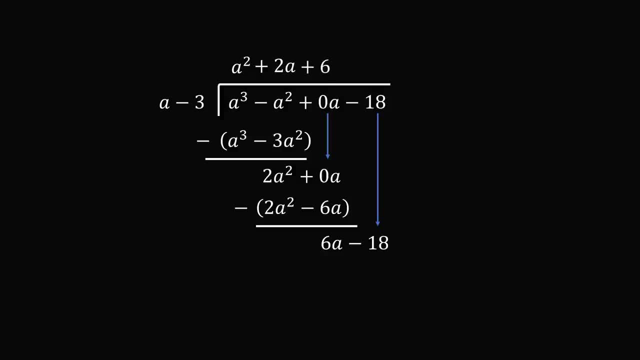 we have to add 6. So we have 6 multiplied by a minus 3. That works out to be 6 a minus 18. And finally, we subtract this, and this works out to be 0. So there's no remainder. 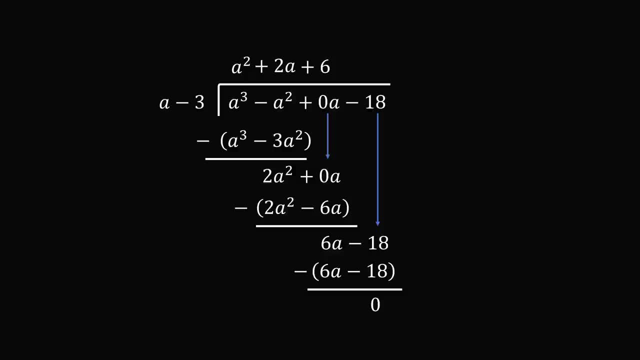 So the original polynomial, divided by a minus 3 is equal to a squared plus 2, a plus 6.. So in other words, a minus 3 multiplied by a squared plus 2, a plus 6 is equal to the original polynomial. Now we want this to be equal to 0.. So that means either a minus 3 is equal to 0,. 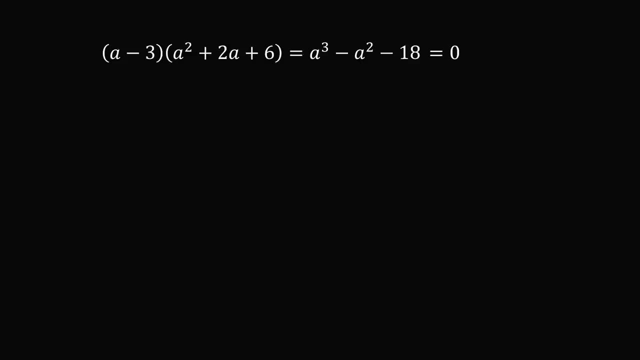 or the quadratic is equal to 0. If the first factor is equal to 0, that means a is equal to 3.. We already knew that. So now we solve this quadratic equation to be equal to 0. We will use Brahmagupta's quadratic formula and we just substitute it in, So a is equal to negative.